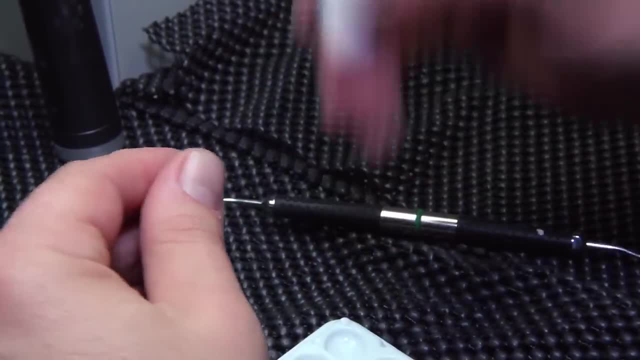 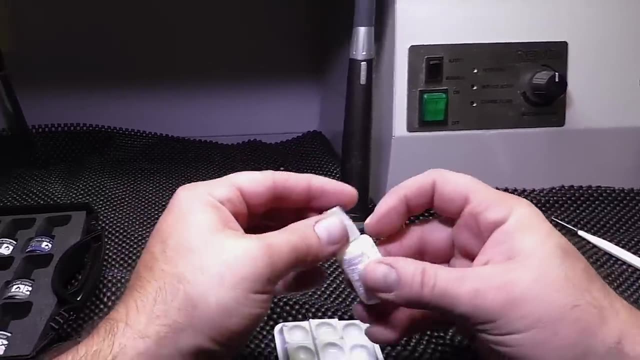 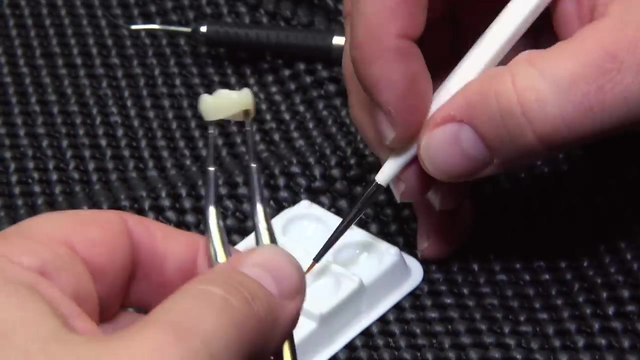 The next step is to take the Ceramic Primer II, and we want to add a little bit into our well here Now. these little palettes come in the Opti-Glaze color kit. We could take our brush, which also comes in the Opti-Glaze color kit, and we apply the Ceramic Primer II all over the surface of. 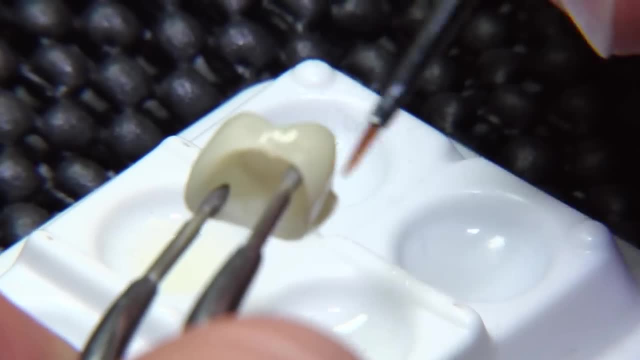 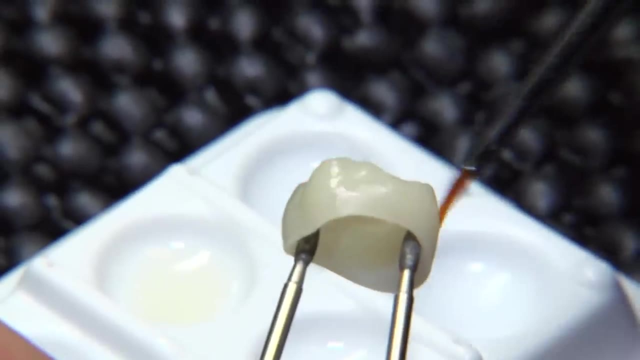 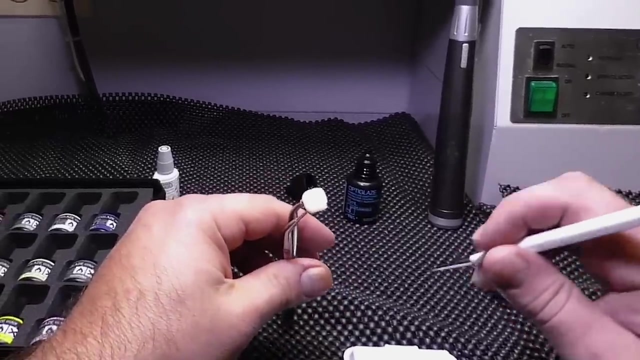 the restoration, just a very nice thin layer, And what this does again is this creates a bond between the Opti-Glaze color and the Cerismart. You can, however, use just the Opti-Glaze color, but one recommended step would be to use this so you have better adhesion. 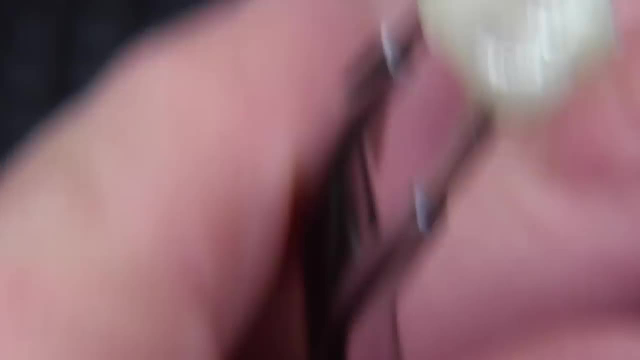 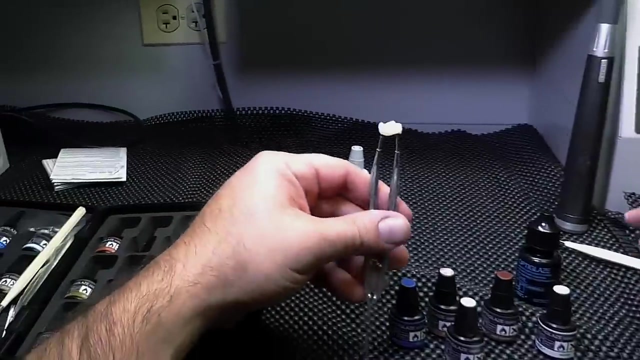 Okay, so when that's done, we could just go ahead and let that air dry, or you can use an air hose to manually dry it. As you see, there are many different shades and colors in the Opti-Glaze color kit. 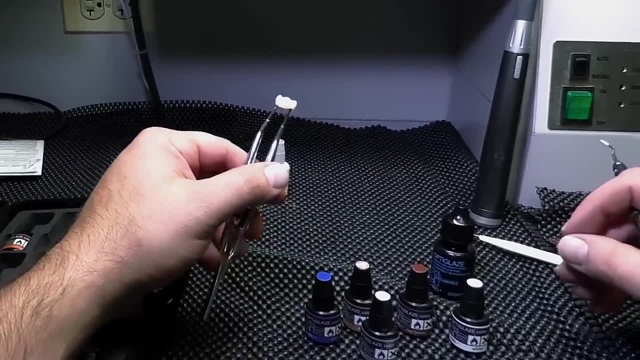 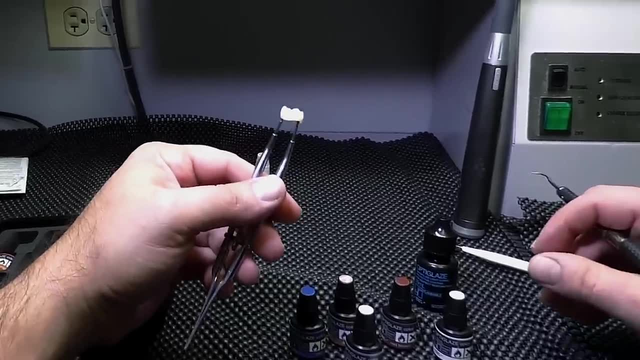 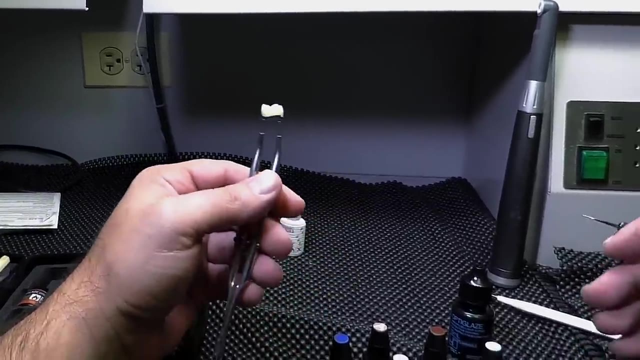 These are meant to be able to achieve subtle and different types of effects. This kit is designed to be used for a process that is as simple as adding one color for warmth, maybe some occlusal stain, to going all the way to full characterization, adding different effects and adding different types of. 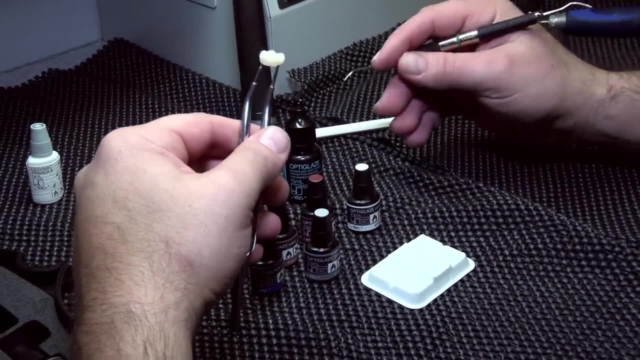 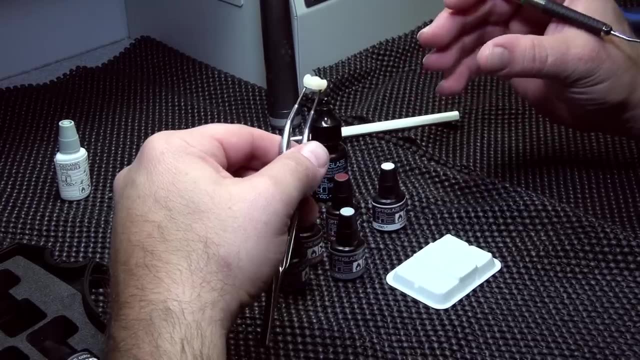 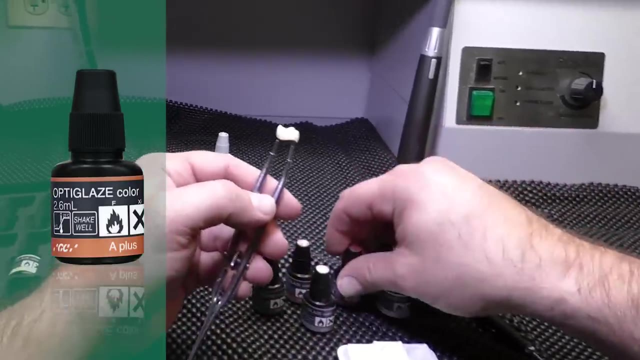 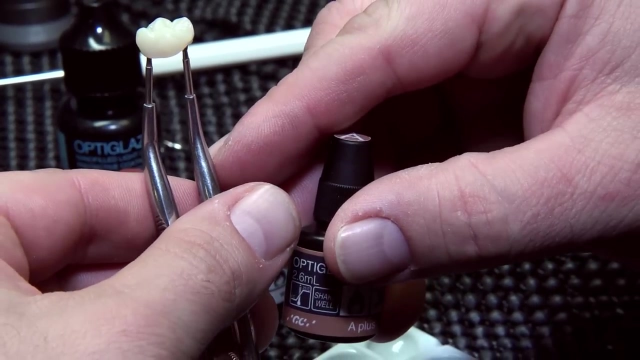 decalcification, There are many different types of applications you can use to achieve the aesthetics, the desired aesthetics, that you're looking for. So, for today's demonstration, what we're going to do is we're going to start off using a little bit of the Opti-Glaze color shade A+. Now, since this is an A-2 Cerismart, 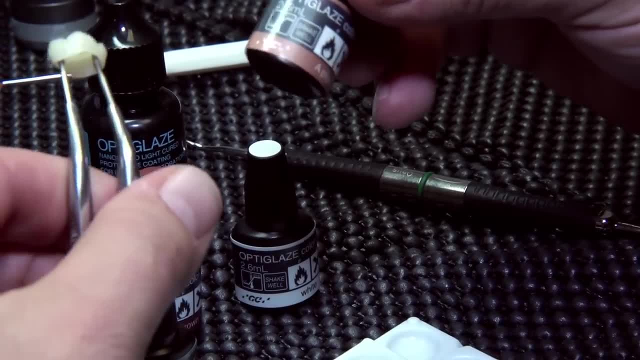 restoration. all we want to do is add some gingival warmth, And we're going to add the didn't correctly寒 create a leading layer today here in the" inequanапtw nested success, and we're going to add the todida plus ona cap vaan1, white of color shadeEuデ分ой visiting out. 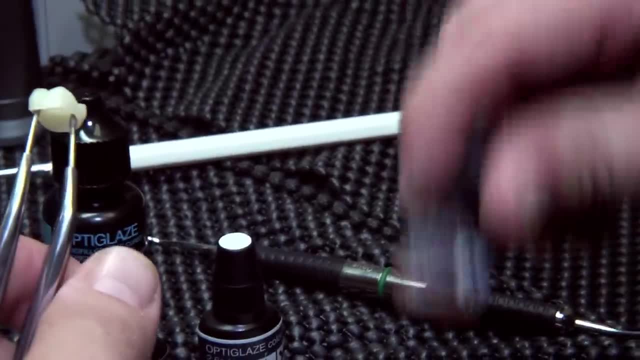 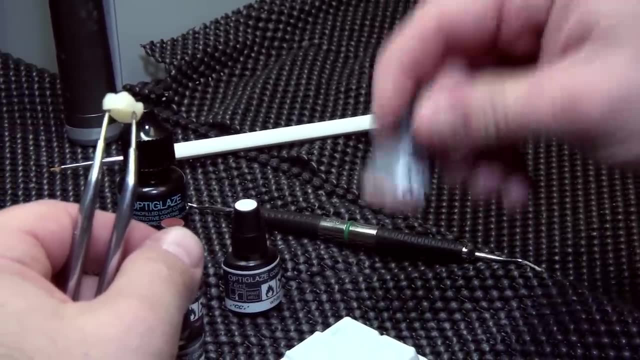 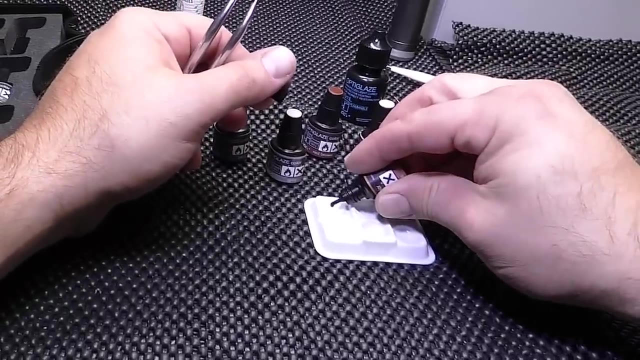 around the gingival and the margin. We want to make sure that we shake the bottle and you hear that ball inside. Make sure we get a good consistency. We could put a little bit of that A shade. A little bit goes a long way. So we put a little of that A shade in. 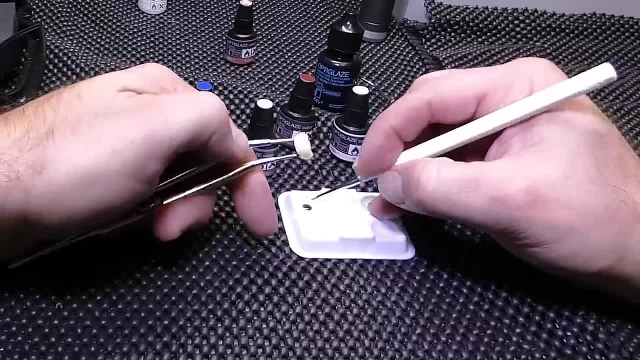 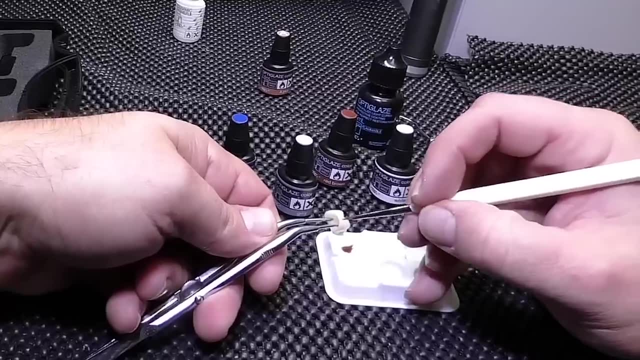 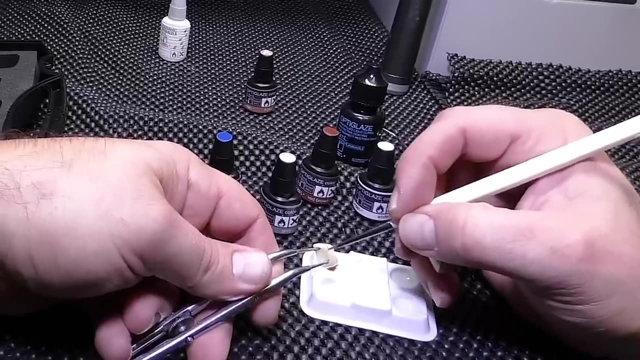 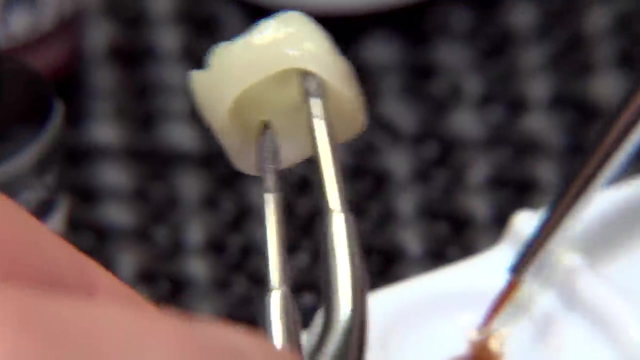 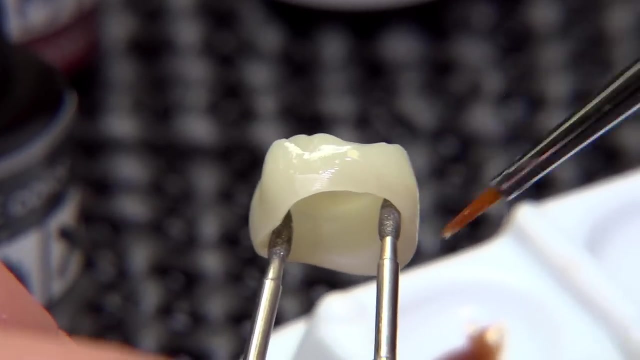 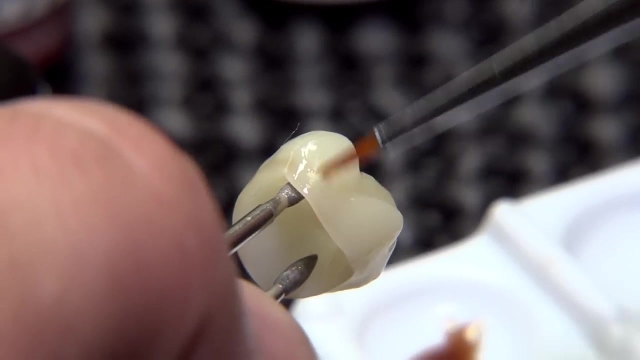 the well And we just start gently going around the margin just to add a little warmth. And again, like I said, a little bit goes a long way. You want to make sure you kind of smooth the color And blend it in so you don't have any extreme lines going on with the color. 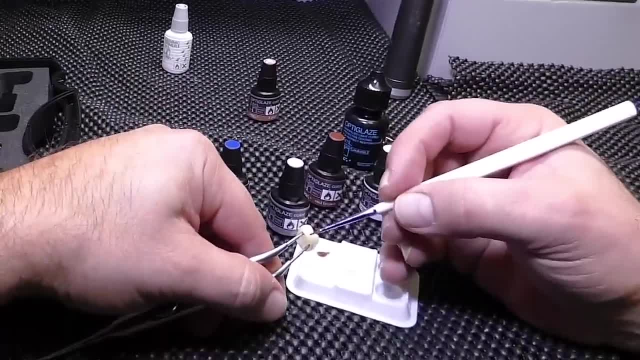 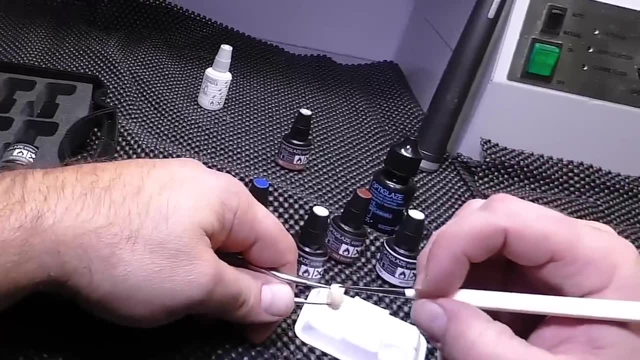 So that's all the warmth that I want right now. I'll maybe put a little bit more here on the buckle, And we're looking for subtlety here- And then we take the light 405.. And then we take the light 405.. 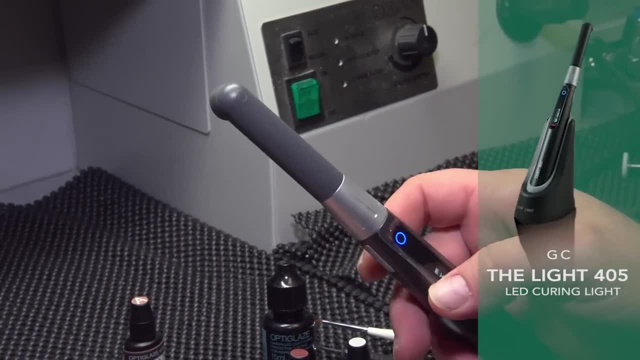 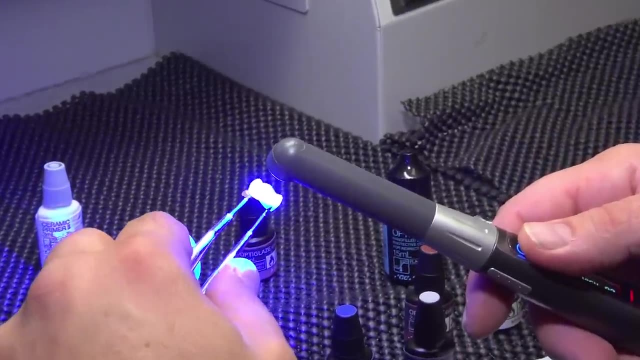 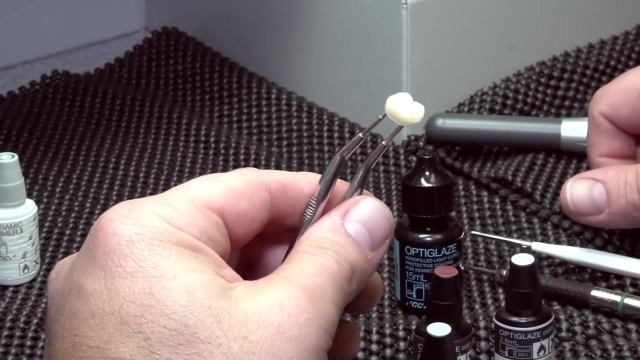 Okay, The light 405 is actually ideal wavelength to cure Opti-Glaze color. I want to make sure we go over the entire surface where we added the shade A. Now for the final cure. we're going to do 40 seconds using the light, But first what we're doing is we're layering our 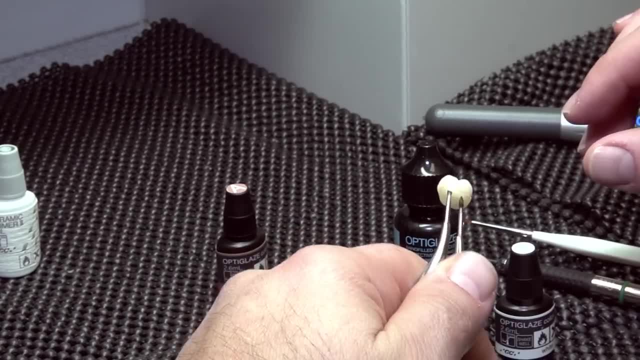 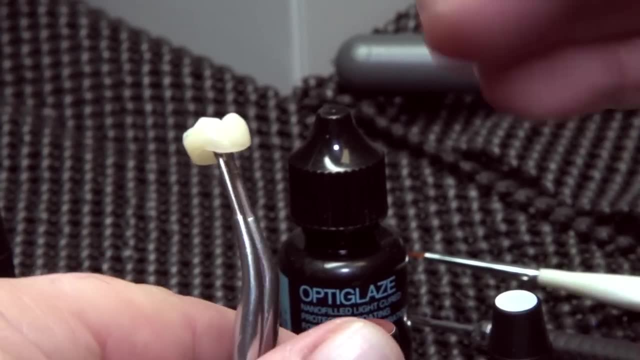 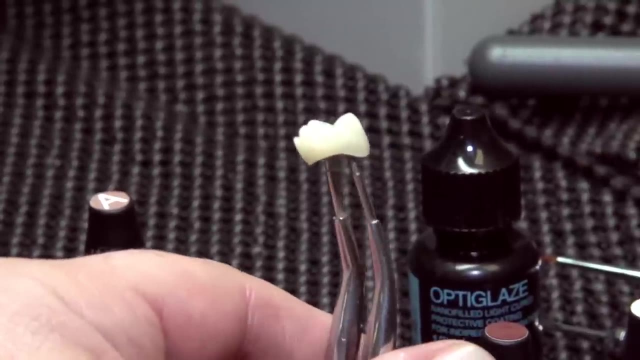 shade, foundation, And as we layer each shade for the effect that we want, we then are going to light, cure each increment. So some may say that this is enough at this point. That's all they may want. But we're going to go now to try and show some stain within the pits and fissures to get that illusion. 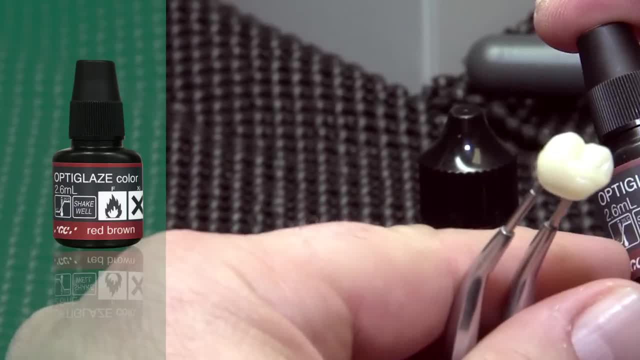 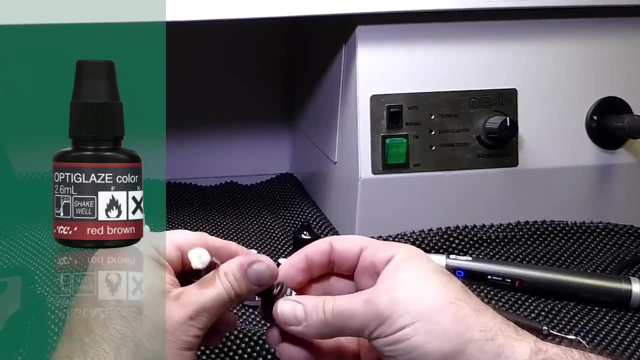 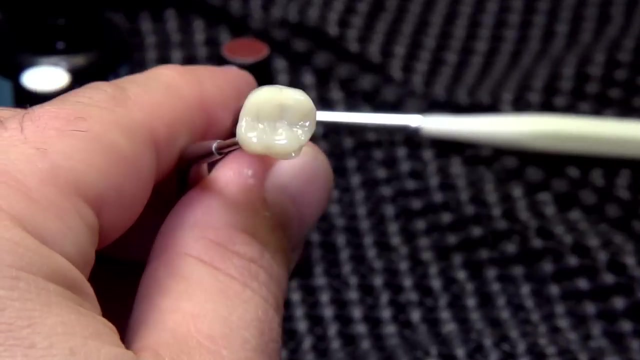 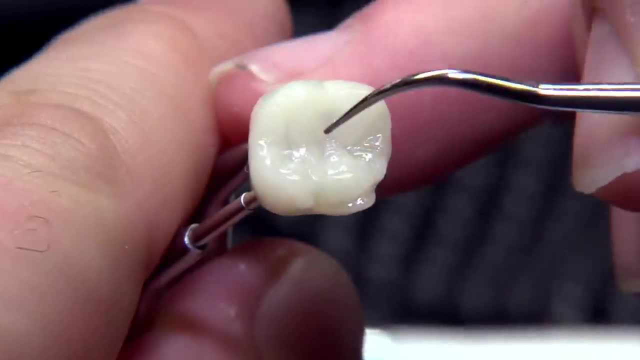 of depth, Maybe not too much. We're going to add red brown for this specific crown. Again, we shake the bottle And put some of this in our well And this is very intense. so a little goes a long way. So we're going to take something like an Explorer And just lay a gentle amount And 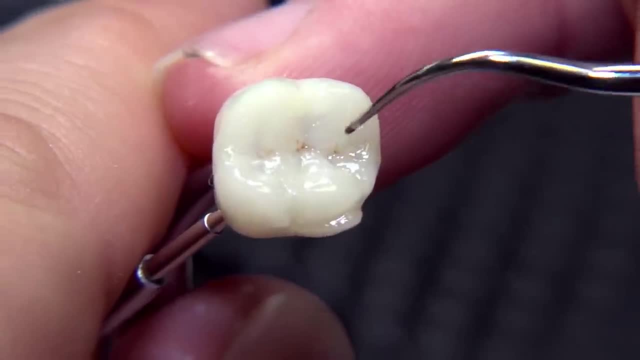 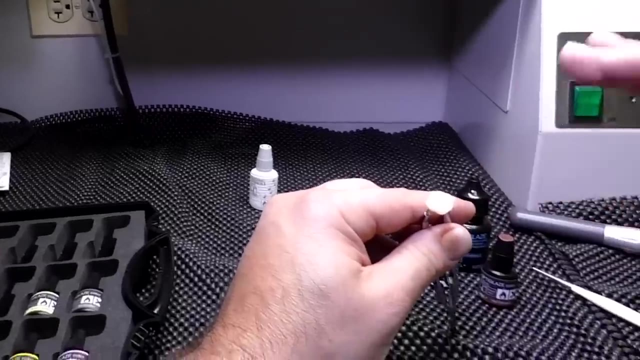 then anything that kind of globs over or puddles. Later on you can take your brush and you can kind of feather that color out and dilute it so it doesn't, So it's not so heavy. And then we're going to take our light 405.. And then we're going to take our light 405. And 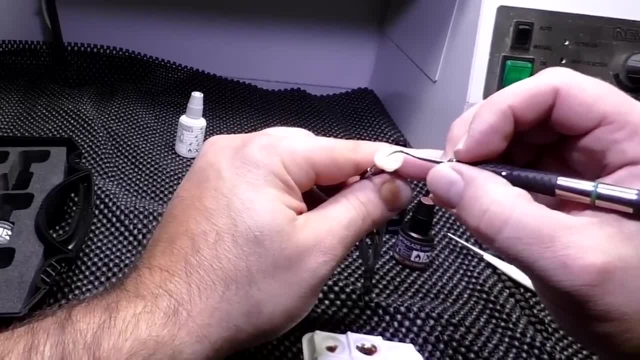 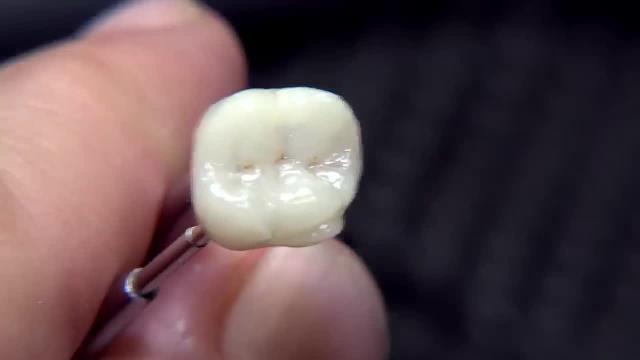 we're going to take our light 405.. And then we're going to take our light 405.. And then here, let me highlight right here- I'm just raising my hand to show it's pretty easy to manipulate in this stage And we don't want to put a whole lot stain in this one. If you're needed to, you could. 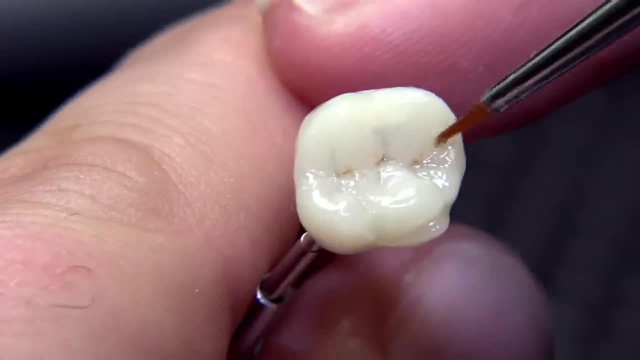 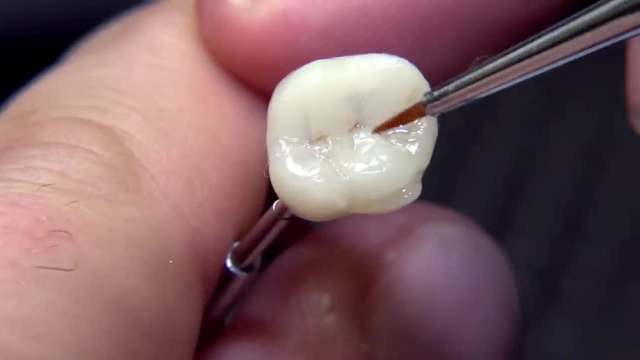 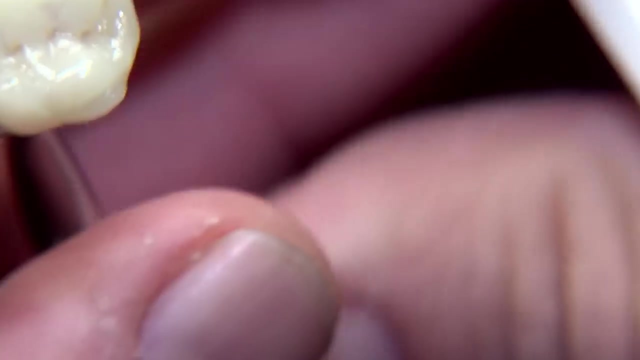 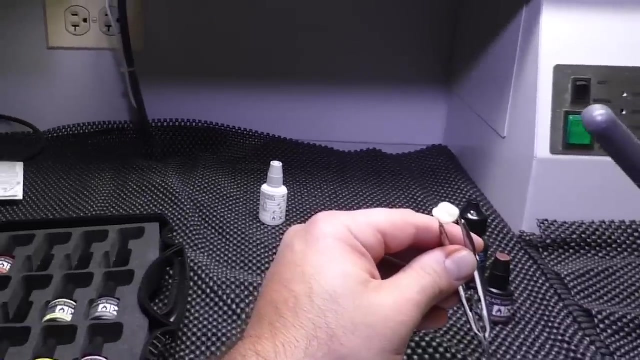 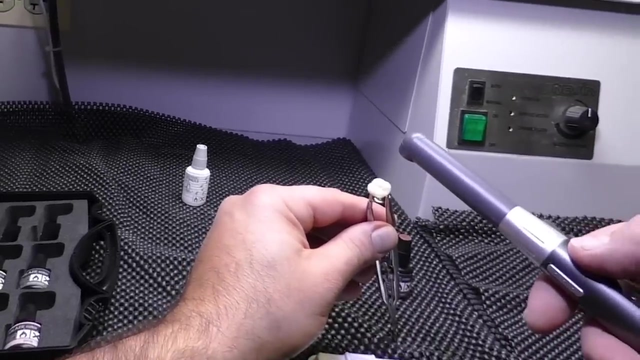 But again something very simple and light Like that, Just enough to add that depth and give some characterization, Feather out any kind of Воah, that kind you crochet puddling. So at this point this again may be enough for some characterization effects. So we're going to take our the light from GC America and light cure. 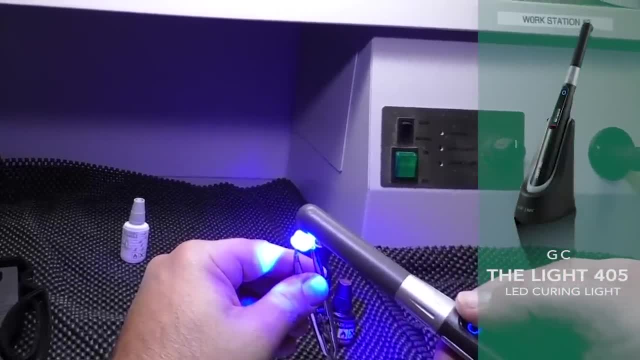 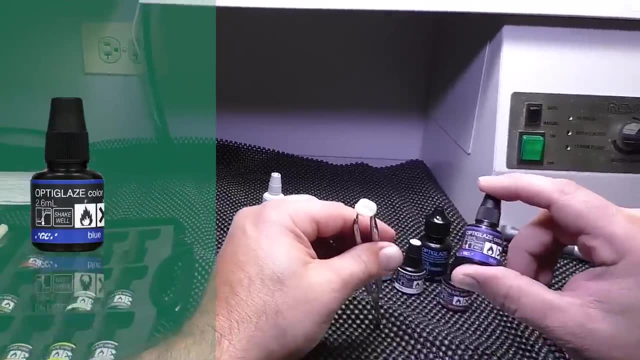 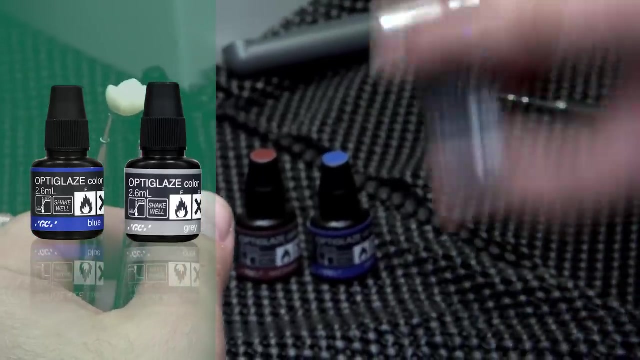 that into place. It should only be a few seconds, because all we're doing is tack curing at this point. Okay, so now, if we really wanted to, we could take the blues and the grays and we'll just go ahead and shake these two up. Now this is. 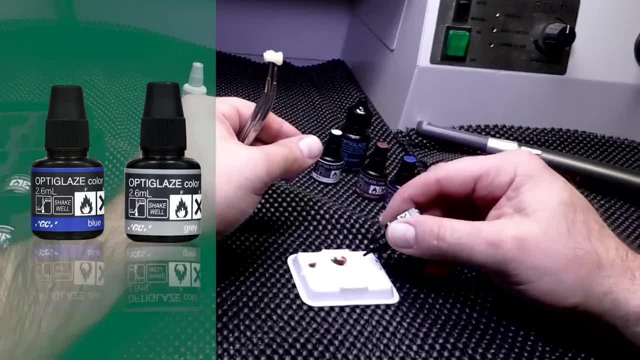 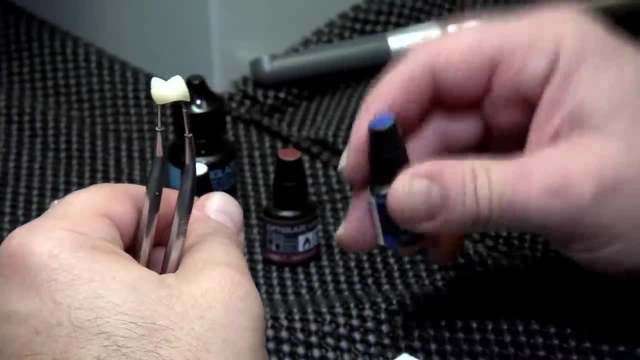 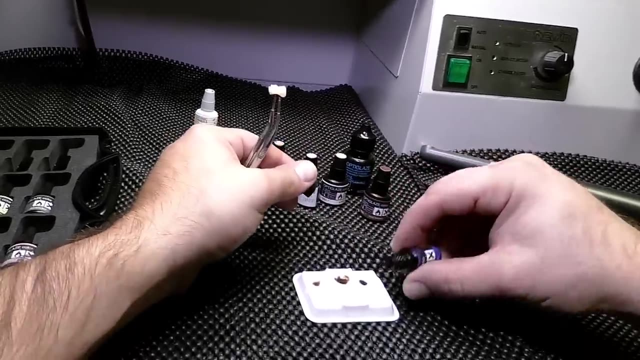 something that will give you the effect of translucency towards the incisal. The only issue is that if you use too much, it is very intense. So this is something you want to gently apply And remove any kind of puddling. So what we can do is, if we need, we could put a. 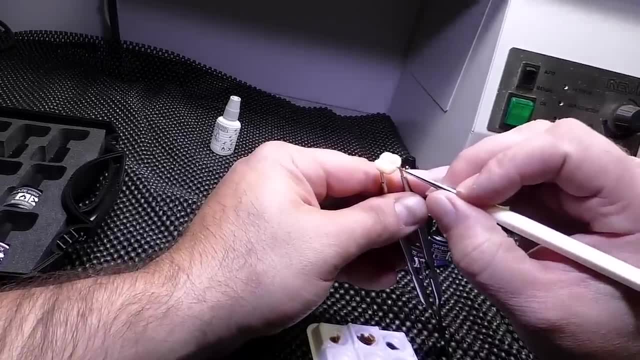 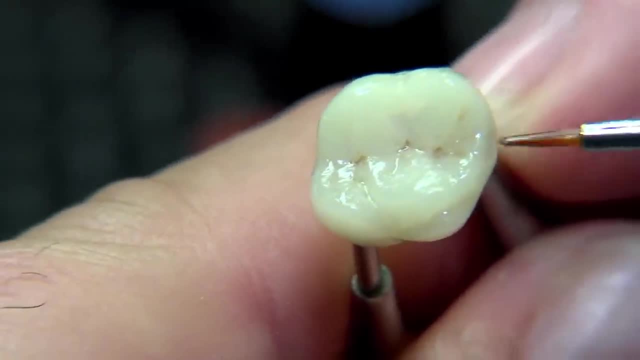 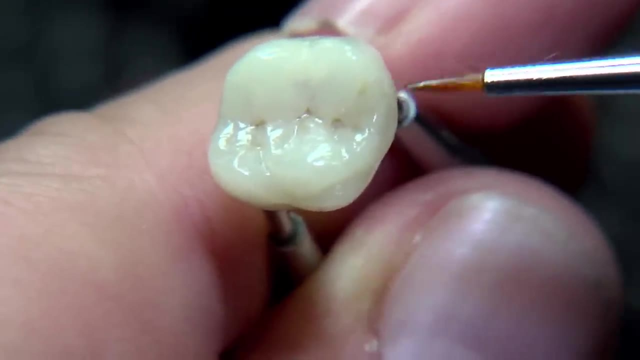 little bit of the gray maybe on the mesial here with the mesial marginal ridge, See, and this automatically gives you that translucent effect. But again, put too much it's going to look too intense. So you can see right away how that kind of gives you that. 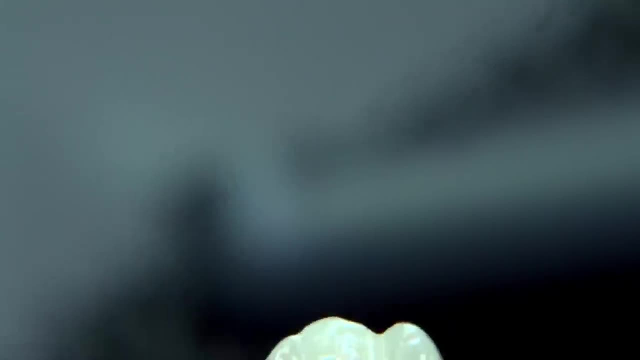 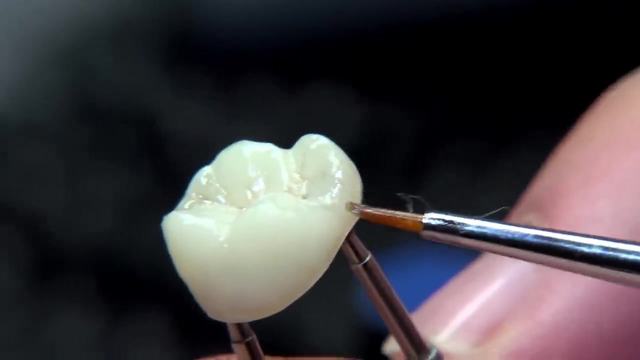 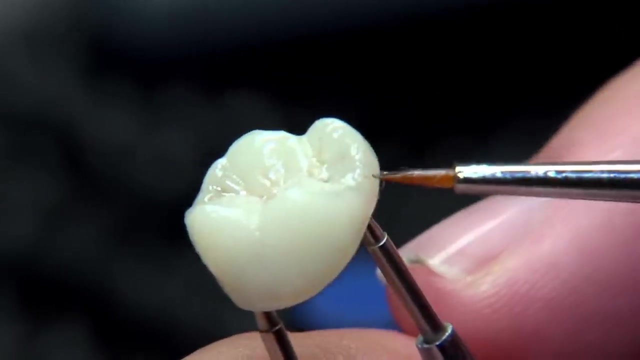 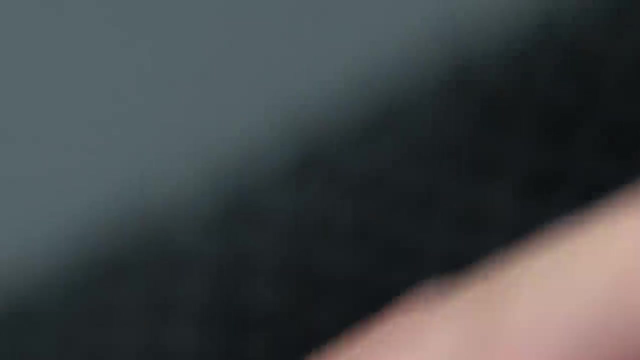 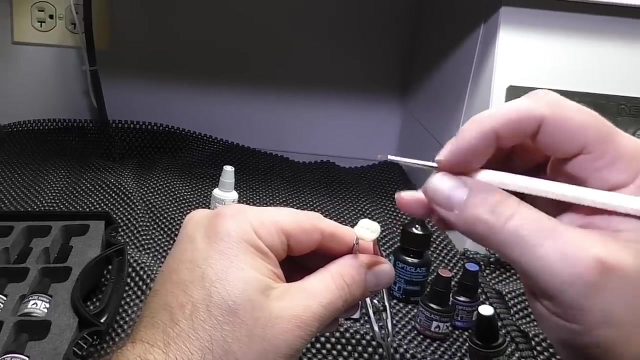 Gives you that effect of translucency. there We can do a little bit on the distal as well, Very gently, And then we're going to go and light, cure that into place for a few seconds. So after we're done applying the grays- and I applied a little bit here in each mesial and 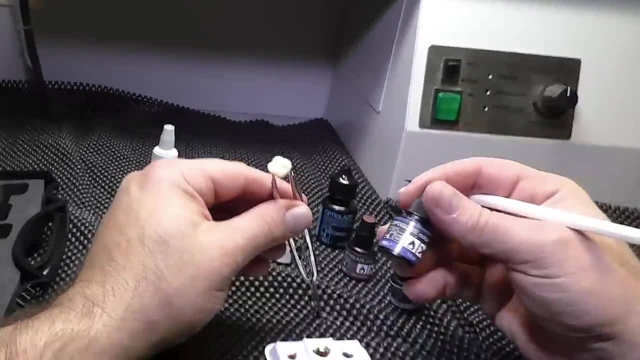 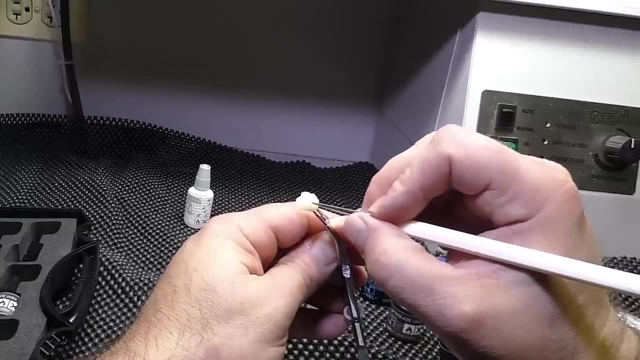 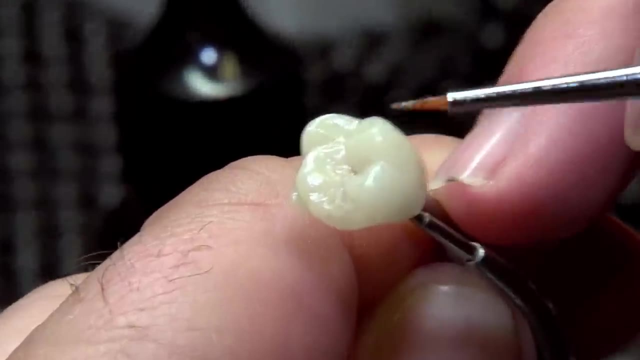 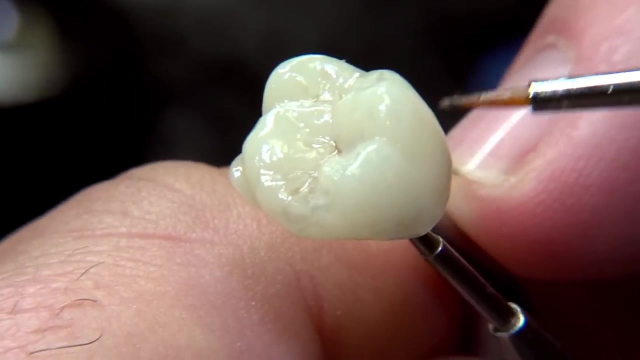 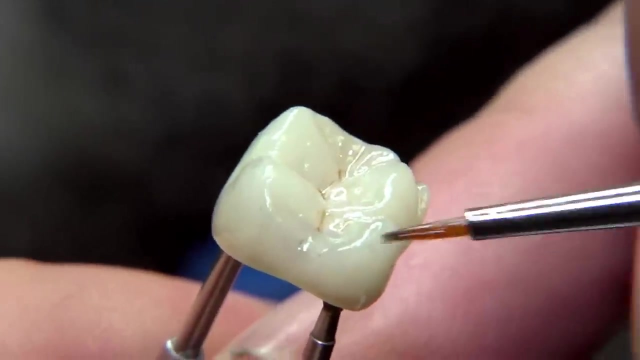 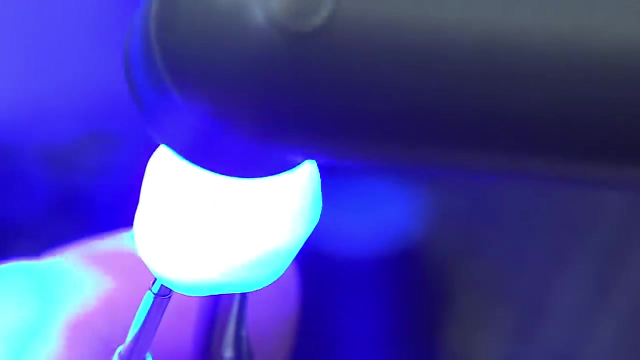 distal marginal ridge. if we want to, we can then take the blue color And basically again very gently, Otherwise it gets way too intense. Just maybe add some kind of enamel effects to the cusps. Once we finish that, we're going to go ahead and light cure again for a few seconds. 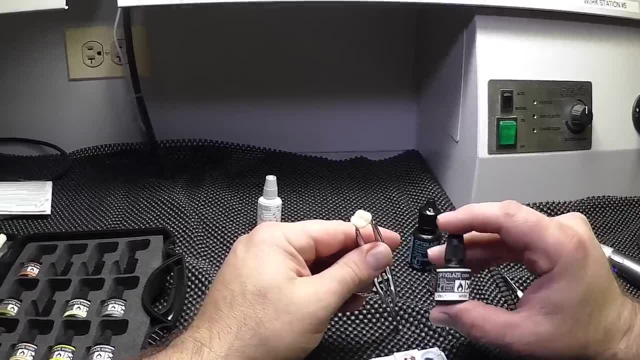 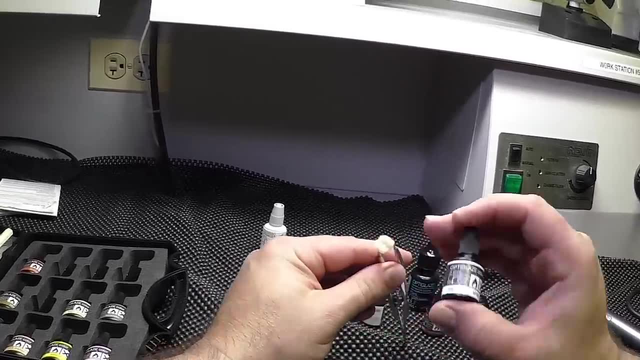 This is a simplified type of application of Opti-Glaze color. Again, we probably did more than typically would be done In most cases. maybe we would add a little bit of the A around the margin, maybe a little bit of the red-brown in the pit and fissures. 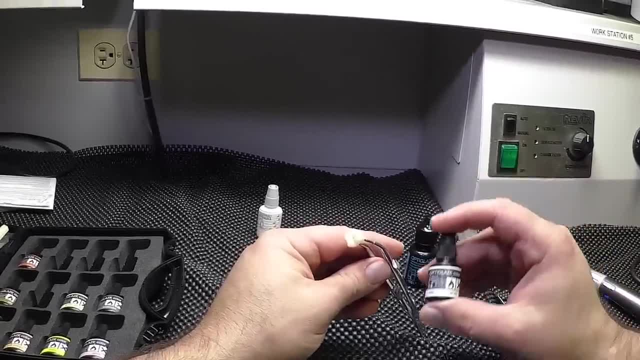 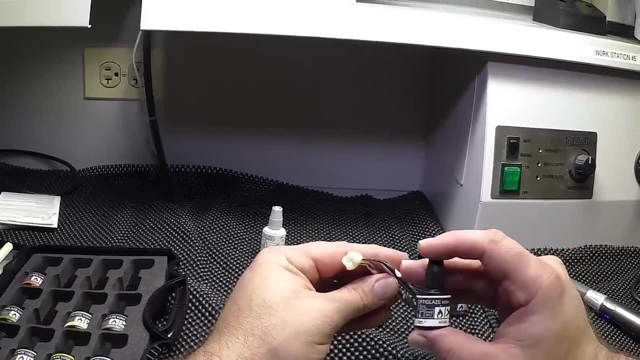 It's optional. You can go as far as you want. You can be as creative as you want with this material. This is just kind of an overview of how this is applied and some of the basic steps you can do to make these Sarismart restorations look really pretty. 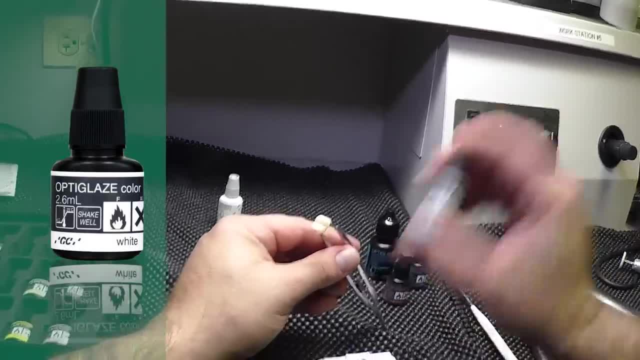 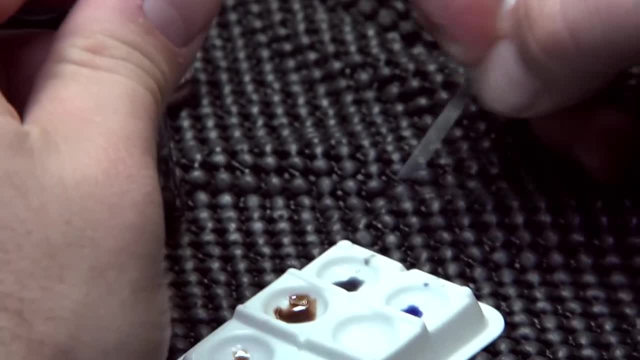 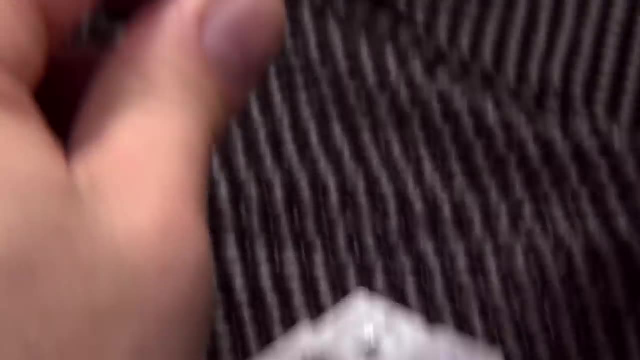 The next step I'd like to do is apply Opti-Glaze color white. Go ahead and mix this up. Now this again: These are pretty intense colors. The point of using the white in this case is just to add a little bit of height to these. 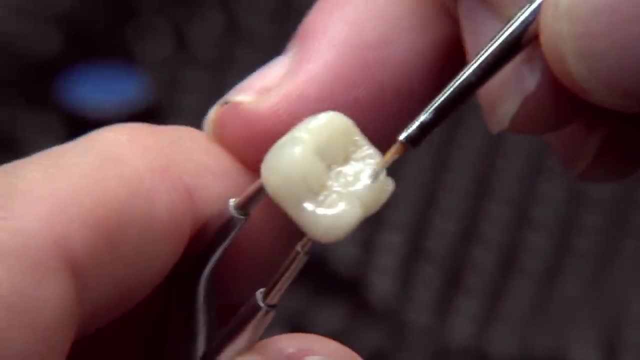 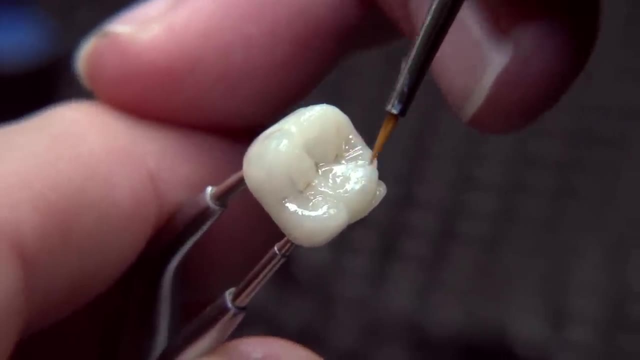 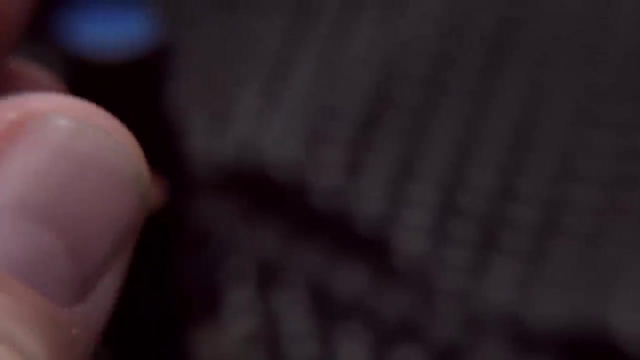 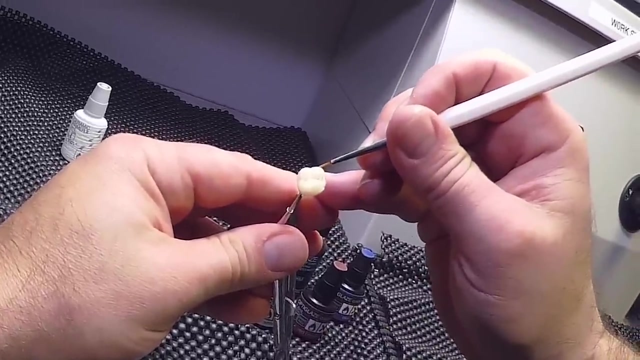 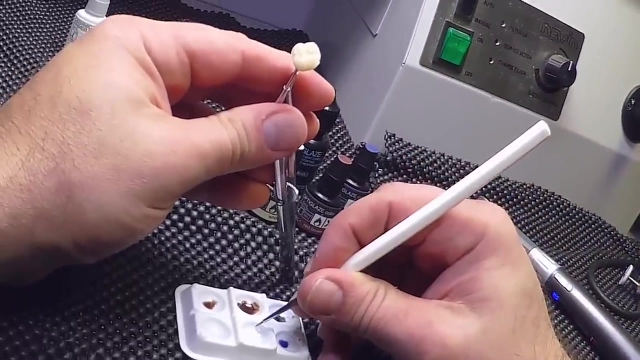 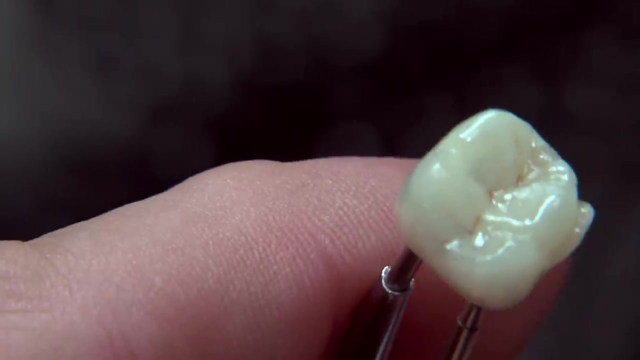 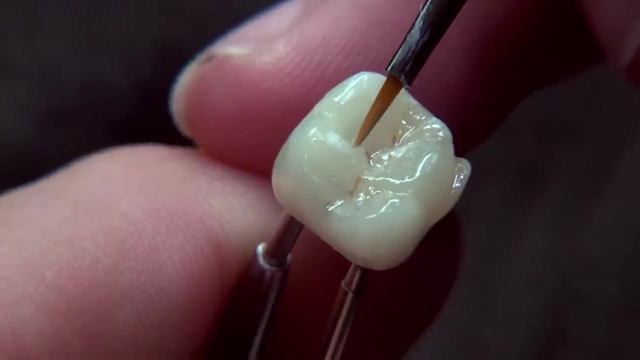 ridges, these cusp tips. Now, they're very intense so you can always brush it away if you need to and blend. There we go, And we're just going to go ahead and go ahead and apply the色 verde. Can you hear me? 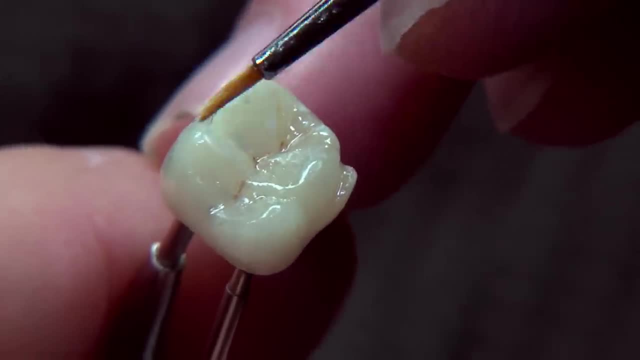 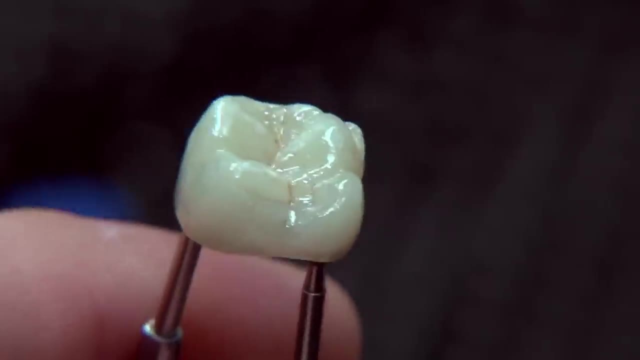 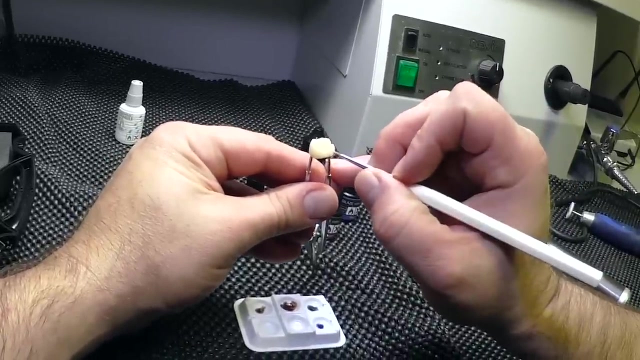 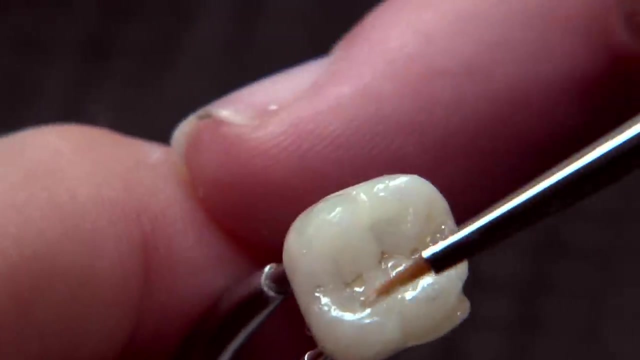 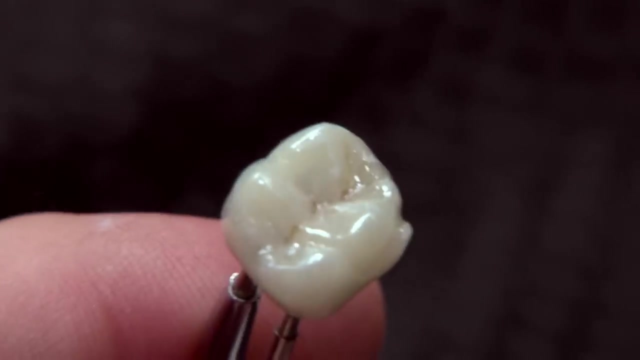 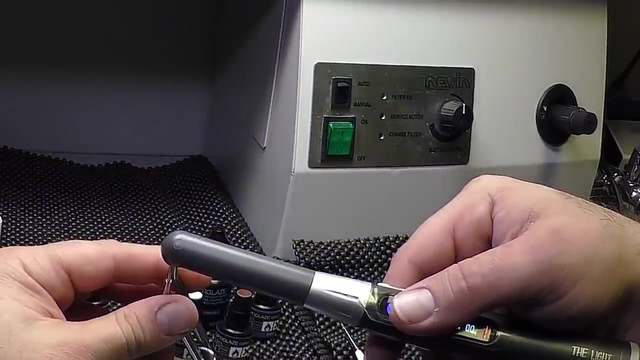 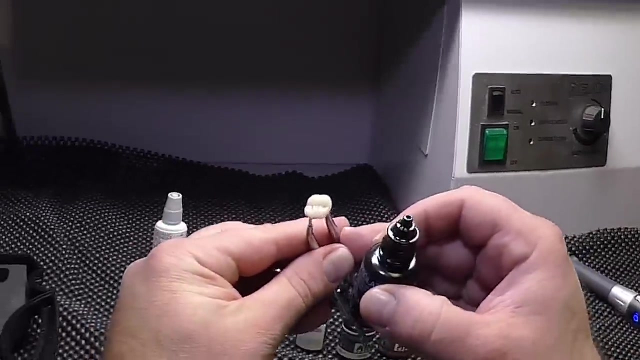 Yes, Try this always: wipe it away. You can really see how it starts to pop. When that's done, we'll go ahead and light cure it for about five seconds. For the last step. we're pretty much done with our characterization. You can see that. 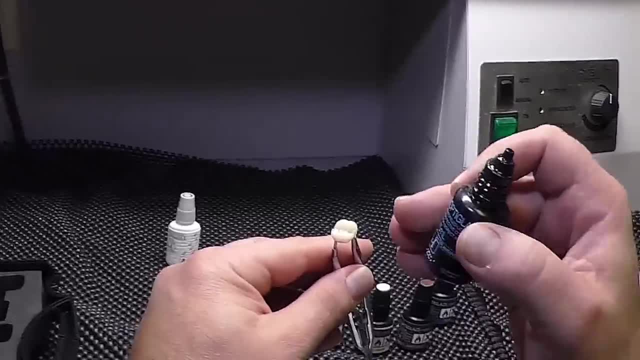 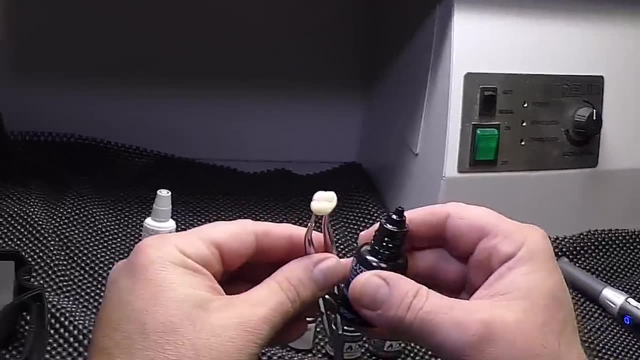 there's some depth there. there's some height- Very subtle, but you can definitely see there's a lot more there than there was when it was first milled out. Now we want to put the gloss on, We want to put that polish on. The way we're going to do that is just by covering. 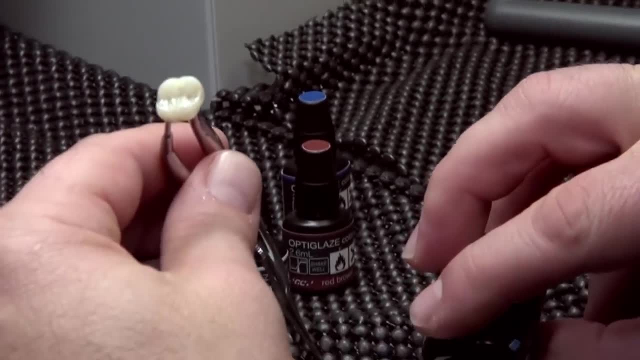 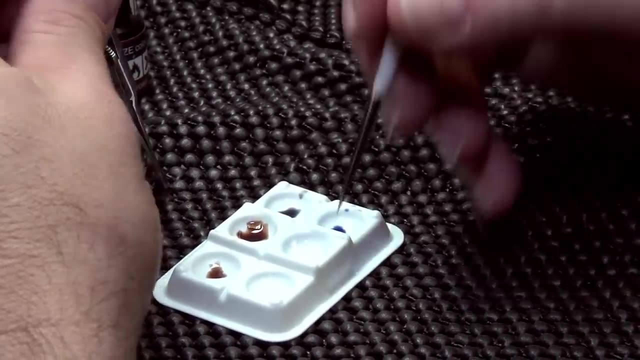 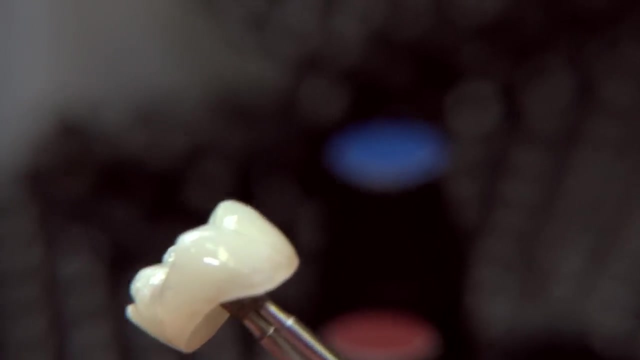 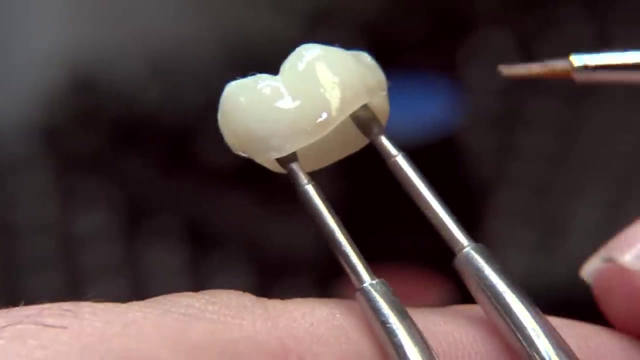 it with the Opti-Glaze Clear. Put a little bit of that in a dish. We're just going to cover the whole restoration with that. That'll give it that real nice glaze. You see, by light curing the colors in place. now they're not running all over the place because they're 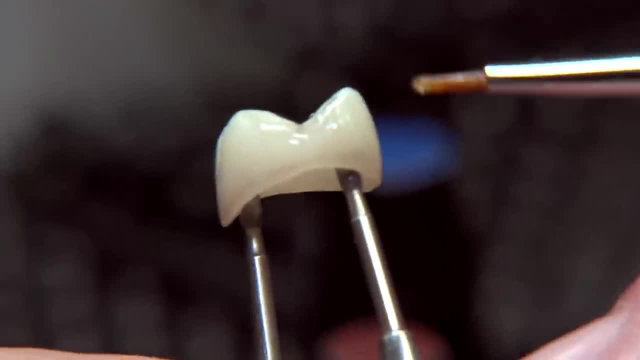 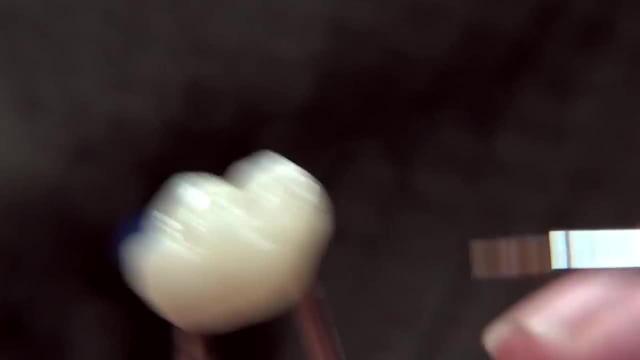 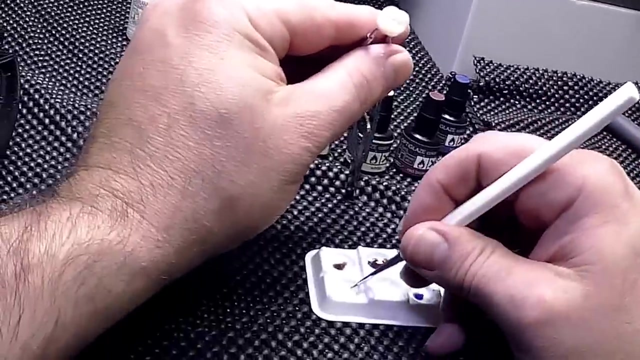 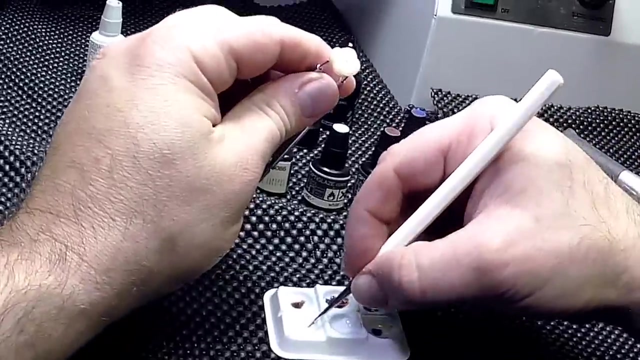 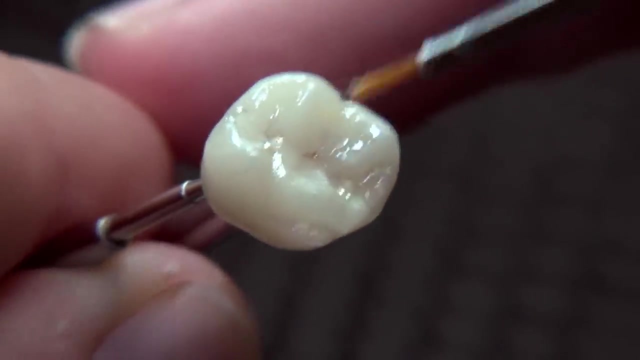 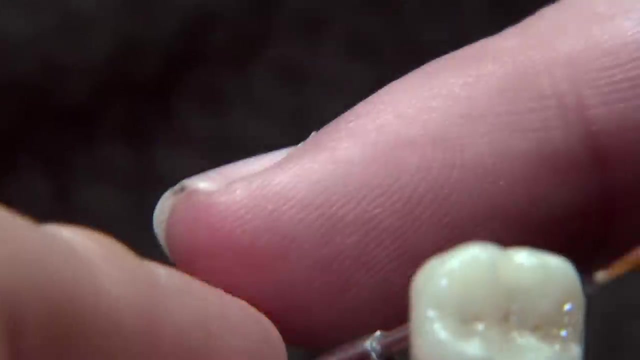 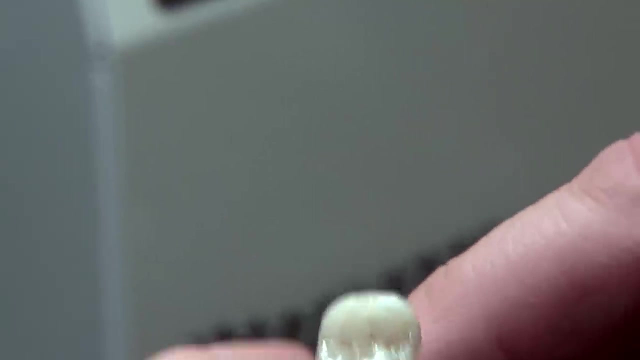 set, Then we're going to put the gloss on and tack, cured On the occlusal. Okay, it's done and ready to light cure. So at this point you can either put it in your light box, if you have one, or if not. 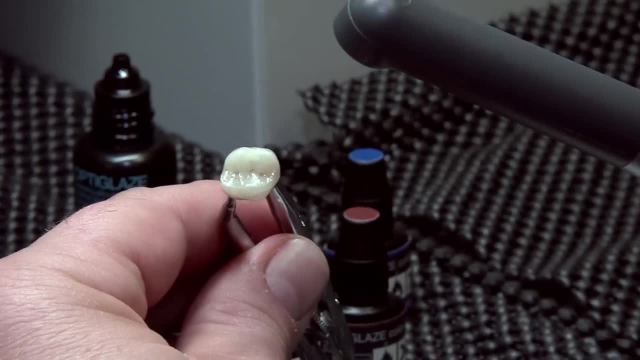 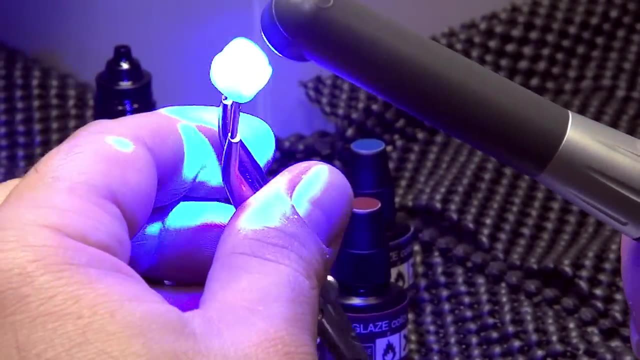 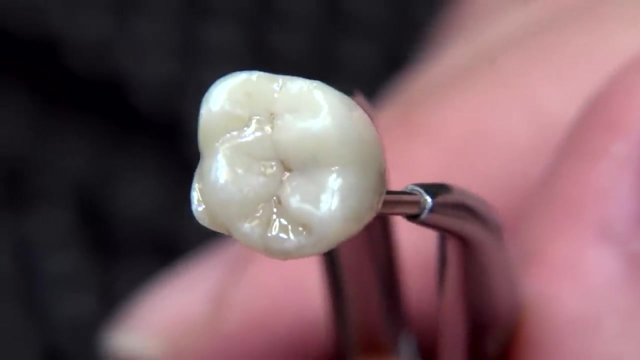 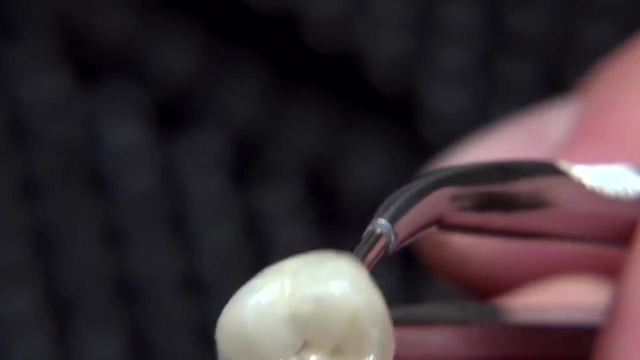 you could take your light- in this case the light from GC, and go ahead and light cure that for 40 seconds, remembering to turn and rotate the restoration to make sure all the sides are equally cured.